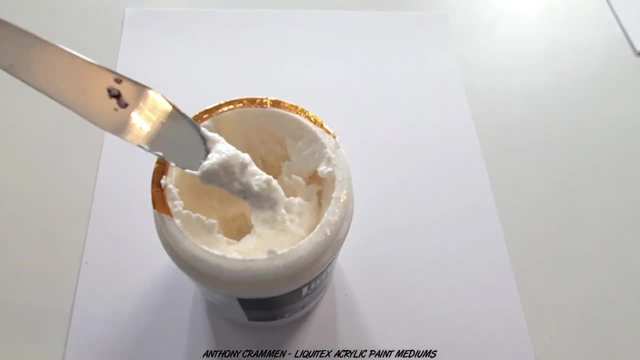 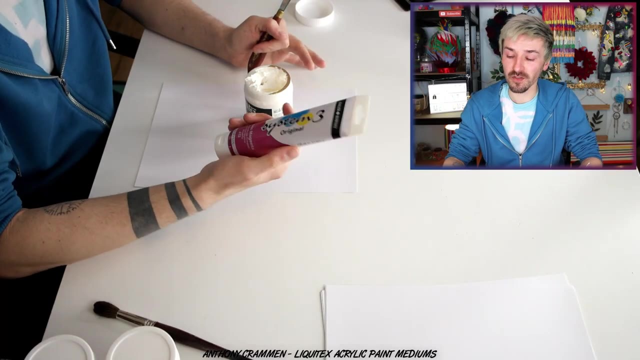 straight away the texture of this: it's almost like a mousse or a yogurt, Quite like a thick, curdled kind of chunky yogurt or something. it seems very light And for all these mediums I'm just going to be using the one colored paint, which is this processed magenta, So I'm just going to use this. 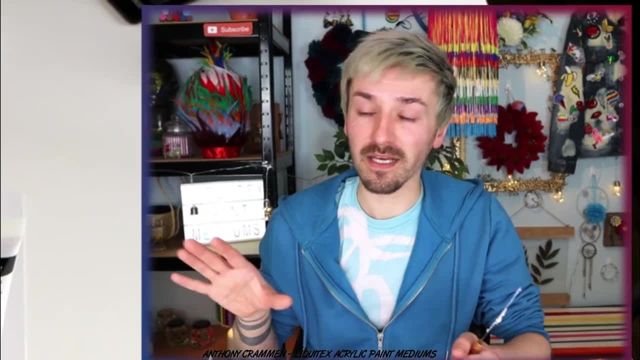 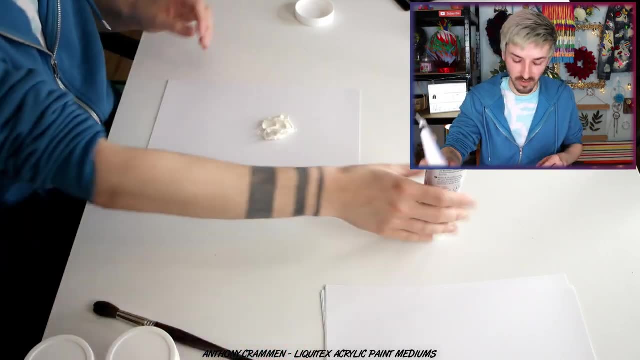 processed magenta. just to give all the mediums a fair chance, make it all, even even though it's not a competition or anything, but just to be fair, All right. so let's have a look, pop that on there and I'm going to add a bit of color to it Straight away. I can see that there's like little. 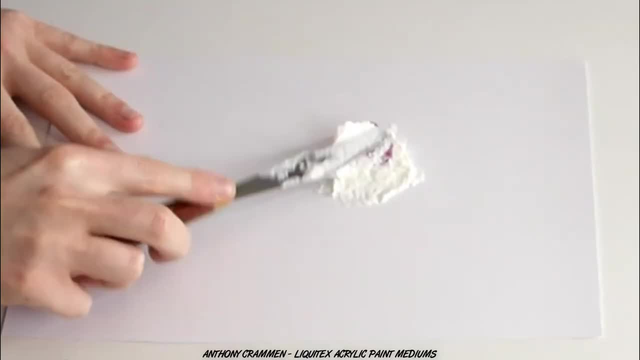 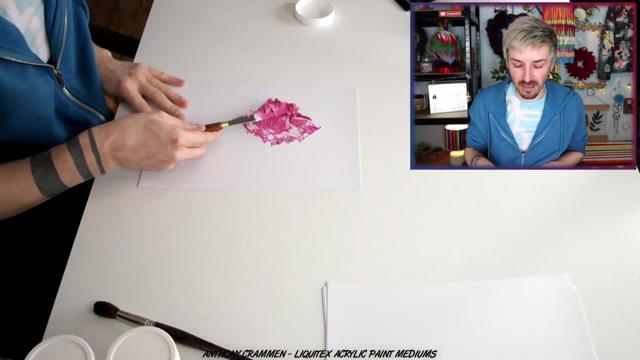 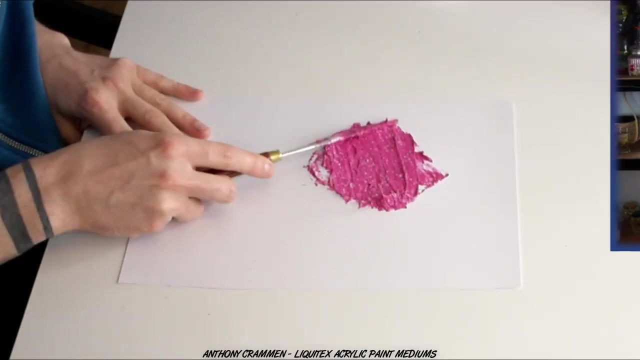 plastic white bits inside **Music**. It definitely does add dimension to the paint. it gives it a thicker consistency and again you can see that there's white flakes in there. It's very subtle, though they're not as kind of obvious, and 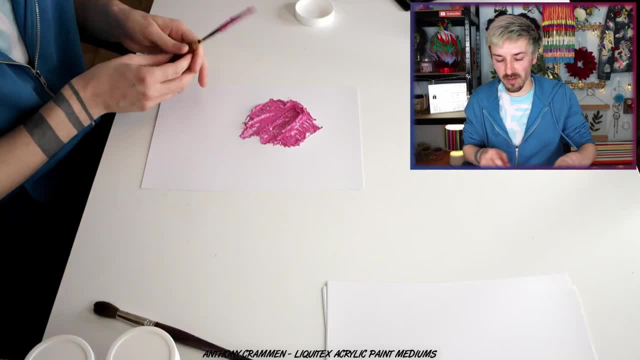 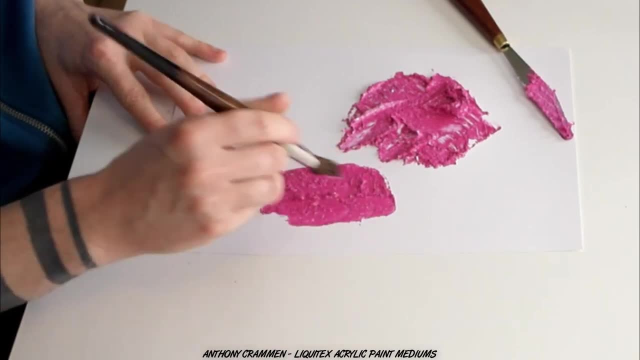 stand out as I would have thought. It seems very interesting. I'm going to try it with a paintbrush as well, just to see what it's like painted. Yeah, it's quite a rough texture, and then you do have those little flakes inside the paint or inside the medium. They don't really show up white once. 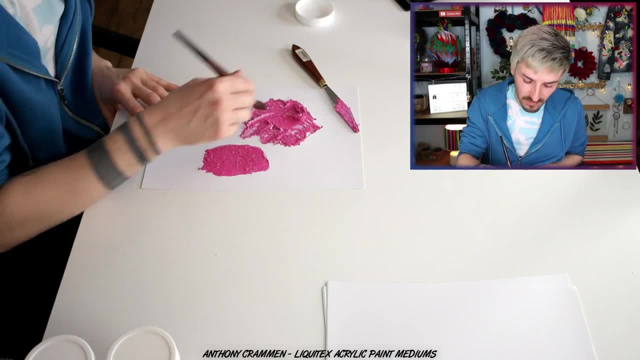 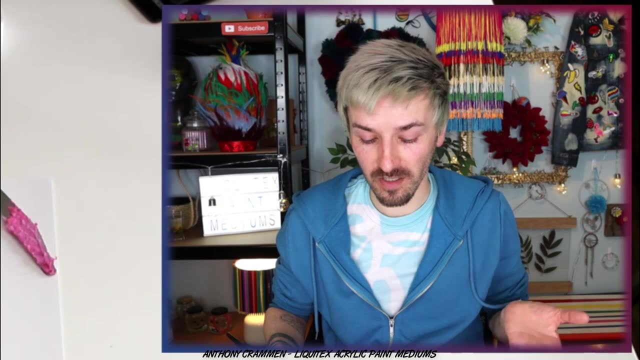 you've got paint on them. they just kind of blend in. So I'll see what they look like once it's dry and maybe they'll kind of show through. It is quite a strange medium. I think it would be good for a little bit more texture. maybe it's a little bit more dimension or a little bit more detail. 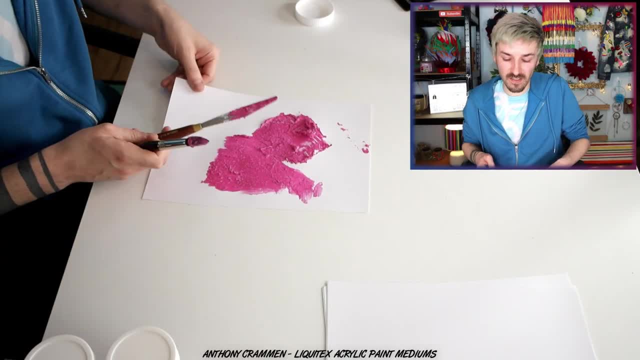 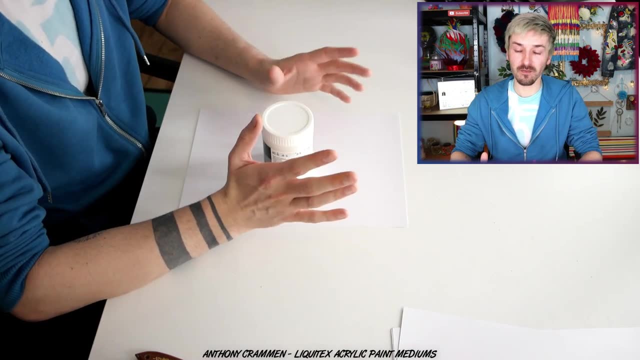 I'm not sure what else you would use it for, Right, so I'll pop that to one side and see what it looks like once it's dry. Okay, next up, we have natural sand, and this is actually the second sand medium that I've got to test out today, because I've got another one as well. I don't know why I bought two. 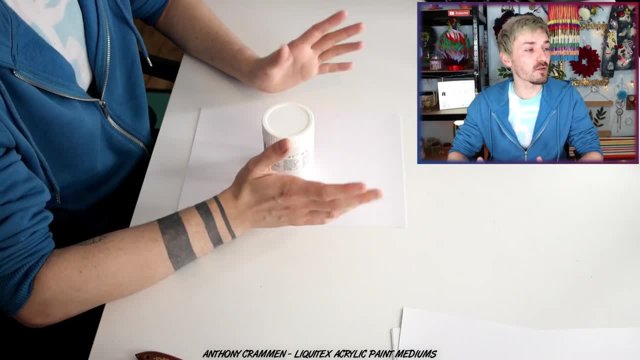 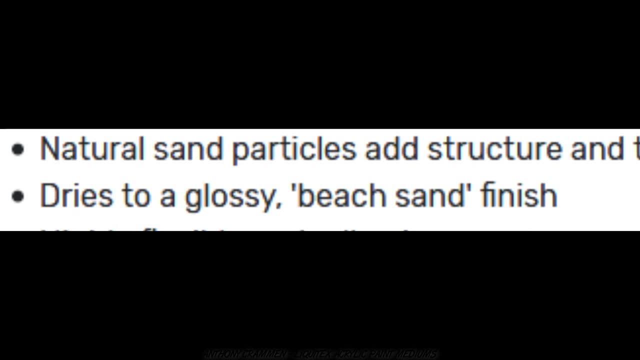 sand based ones, but I did. It does say on the website that natural sand particles add structure and texture to this a hundred percent acrylic polymer gel. It dries to a glossy beach sand finish. It's highly flexible and adhesive. it will not chip or crack on canvas. It gives an opaque. 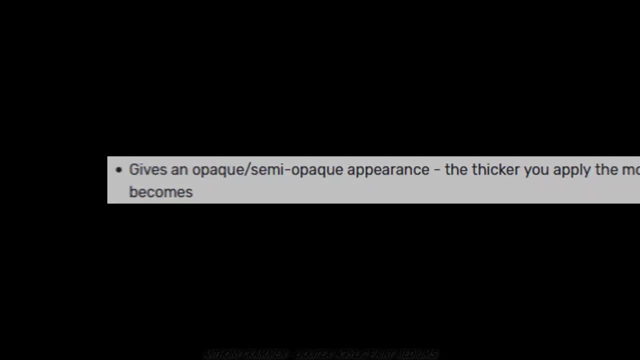 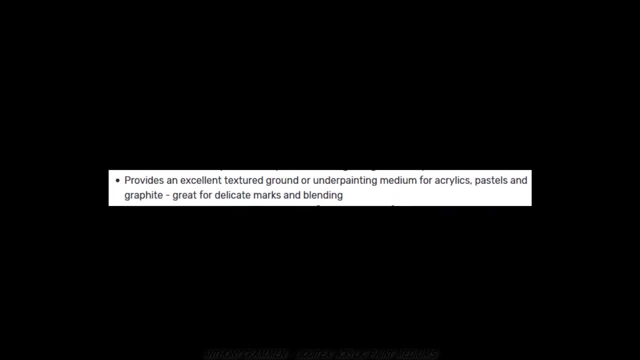 semi-opaque appearance. the thicker you apply, the more opaque it becomes. It can be used on its own, mixed with color or over painted. once dry Provides an excellent textured ground or underpainted medium for acrylics, pastels and graphite. Great for delicate marks. 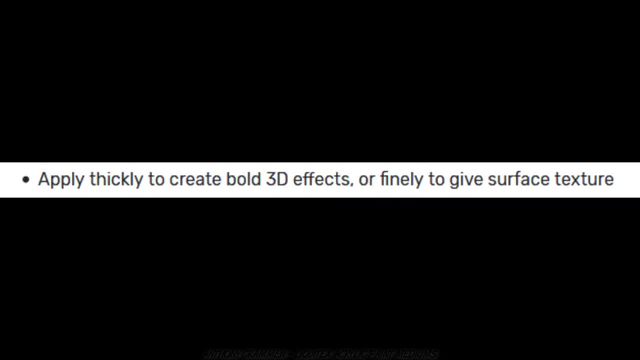 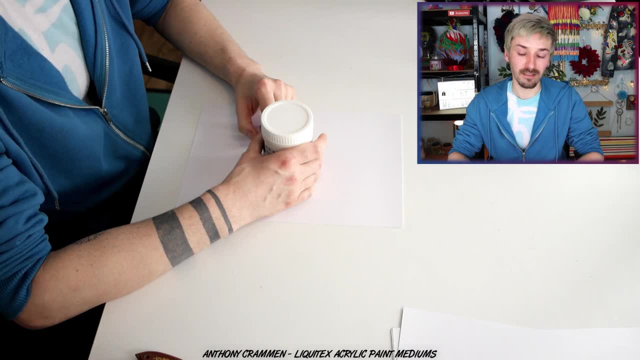 and blending. Apply thickly to create bold 3d effects or finely to give surface texture. I'm pretty sure it said that about the last one. Maintains color adhesion, durability or quality. It said that about the last one as well. just repeating yourself? All right, let's. 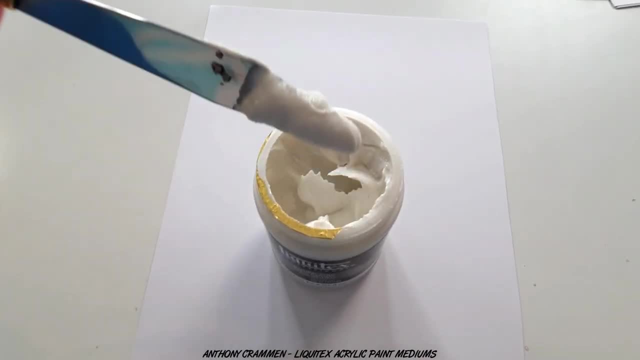 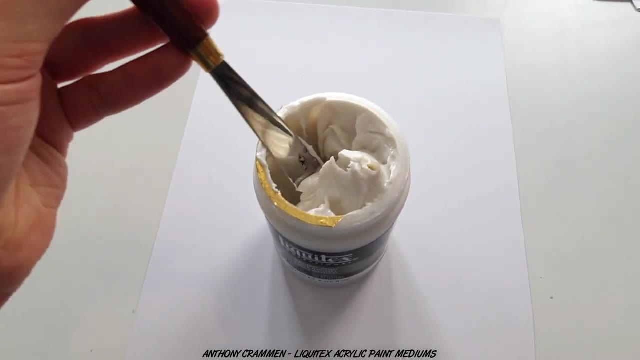 open it up see what it's like. Okay, so this one is quite smooth. it's very gel-like and I can feel that roughness from the sand. It doesn't have any color to it, it's very just white. So we'll see. 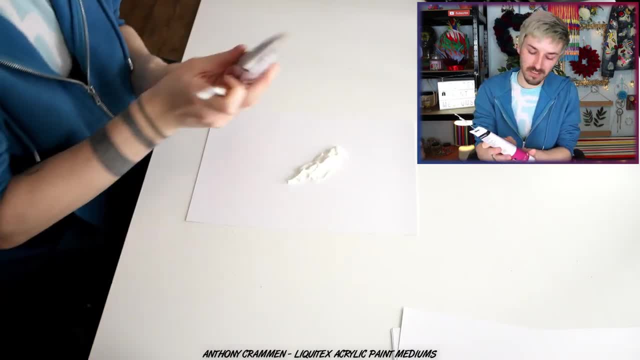 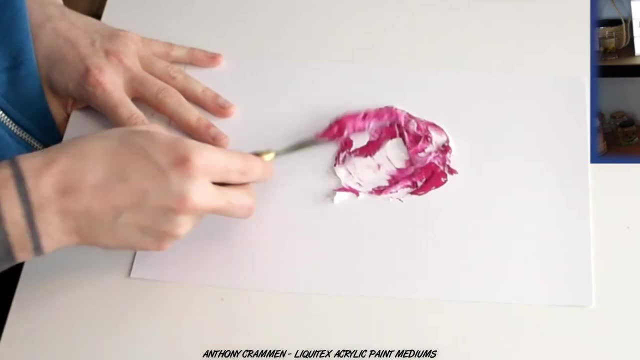 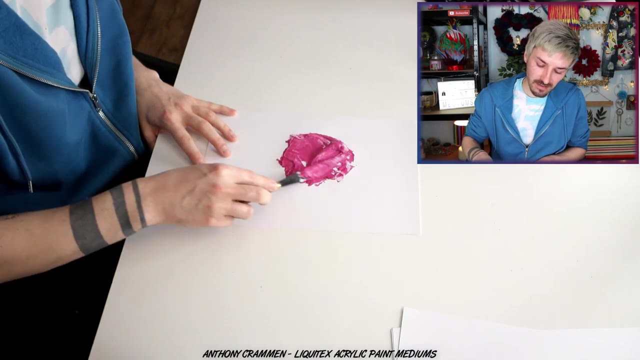 what it looks like. we'll just add a bit onto this paper here and we'll mix a bit of our paint in **Music**. It definitely adds more texture and I can imagine it's quite buildable. I think you get some very nice. 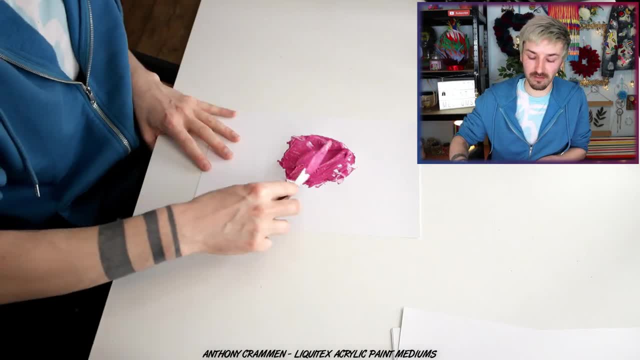 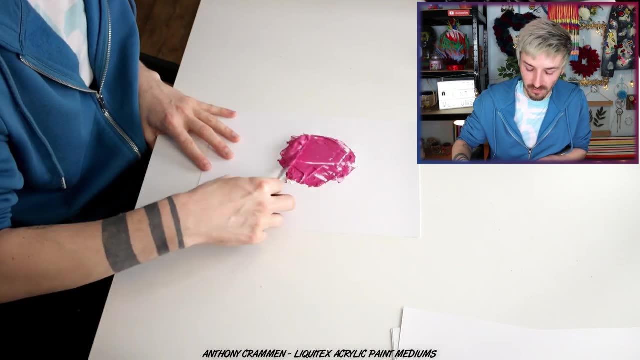 thick effects with this, and if you hear it- I don't know whether you'll be able to hear it- You can kind of hear that sand in there, so it's interesting. It hasn't changed the color of the paint too much either. let's try it with a brush. Okay, it's quite nice. it just feels like I put. 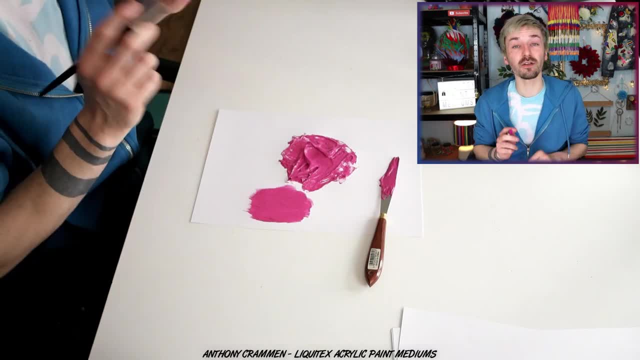 sand in my paint, so that's not bad. I don't mind it, But we'll see what it looks like when it's dry. So since we just did natural sand, I thought we would do resin sand next, just to see if they're. 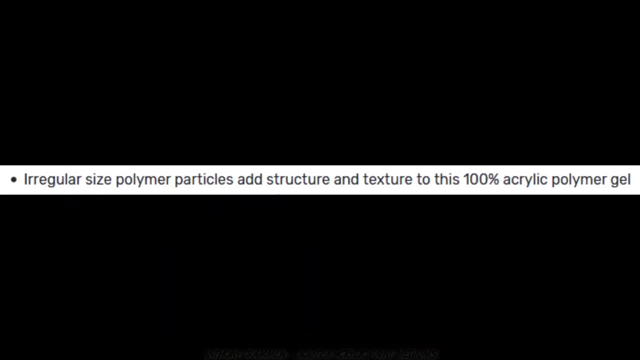 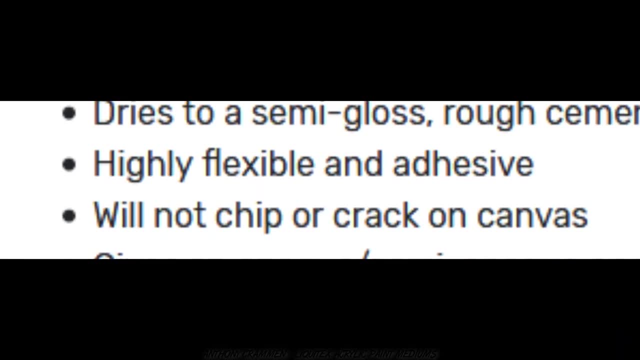 different Right. so on the website it says that a regular size polymer particles add structure and texture to this 100% acrylic polymer gel. dries to a semi-gloss rough cement finish. highly flexible and adhesive. will not chip or crack on canvas again. Gives an opaque, semi-opaque appearance. 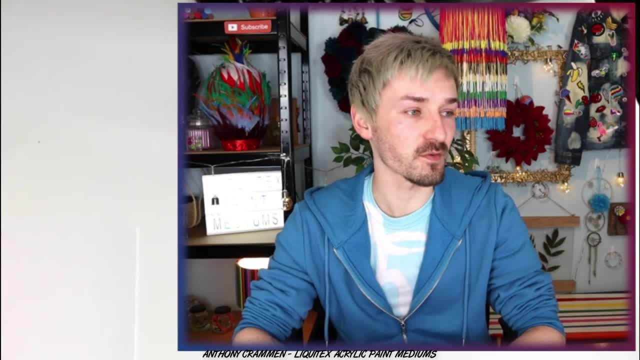 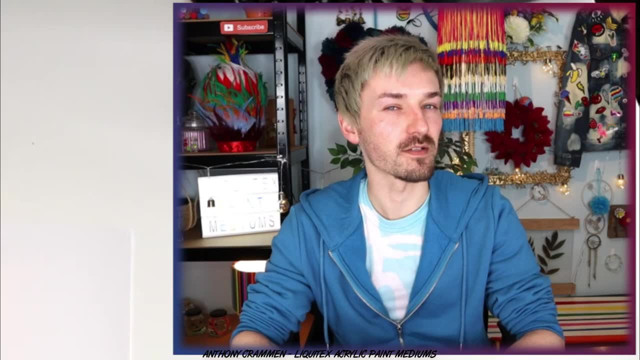 the thicker you apply, the more opaque it becomes. It said that about the last one as well. Provides an absorbent, granite-like ground when mixed with black lava and ceramic stucco, probably pronouncing that wrong. Ideal for soft body acrylic application. 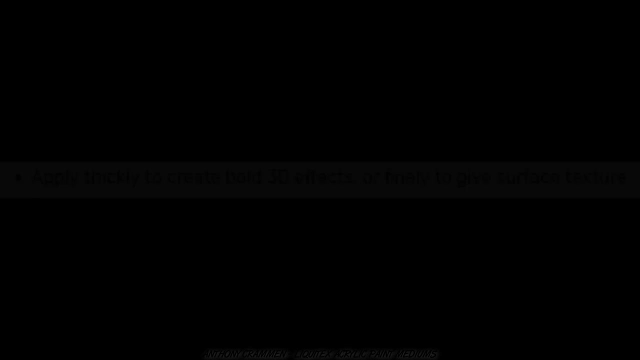 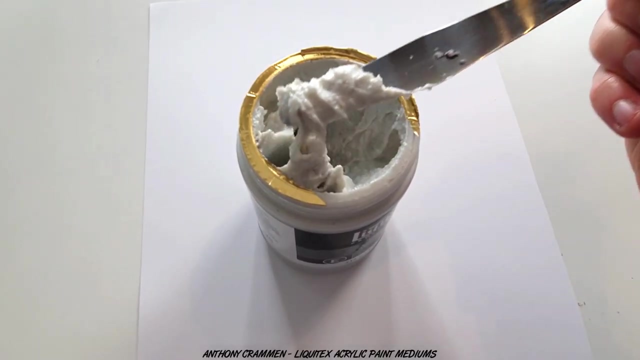 Apply thickly to create bold 3d effects or finely to give surface texture. yeah, it's just repeating what it said about the last one. Okay, let's open it up, see what it's like. Okay, it definitely seems like a thicker medium than the natural sand one. the other one was very kind of not runny, but gel. 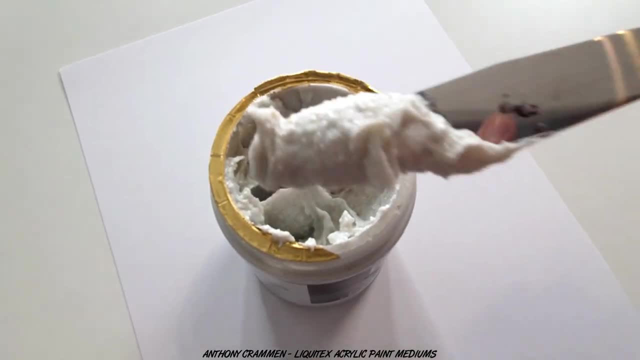 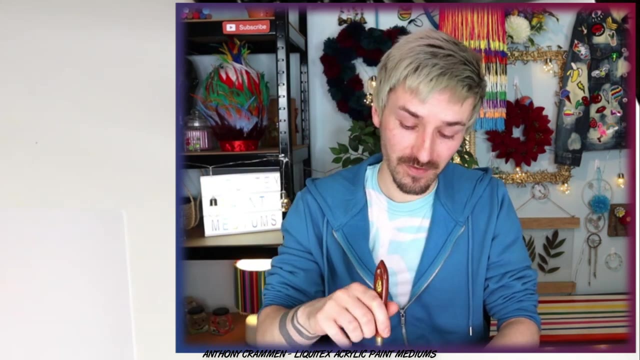 like, and this one is more kind of thick and structured. And, by the way, if my voice sounds really croaky, I've had flu for about two weeks now and it's just not leaving us alone. So if I sound a little bit rough, that's why I wasn't out on the lash last night. 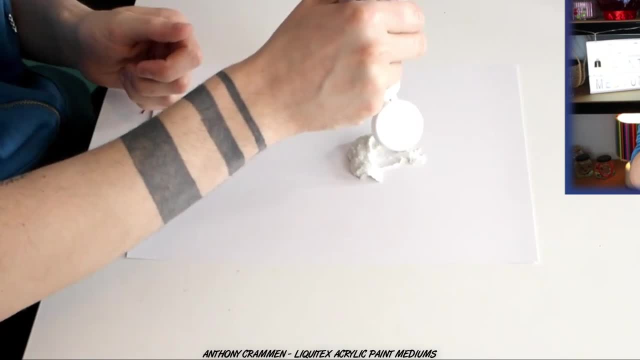 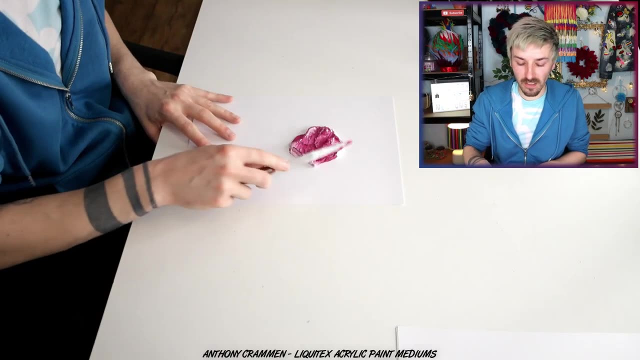 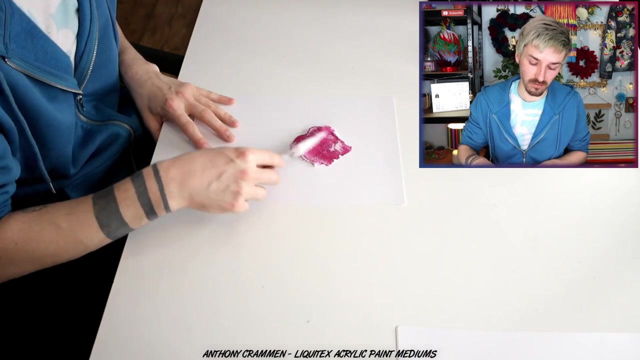 All right, let's mix it with some paint. see what it's like. **Music**. Okay, straight away, I can tell that the sand particles in this one are a lot thicker, or a lot bigger than the natural sand one. The natural sand was a lot finer and I think this one would be. 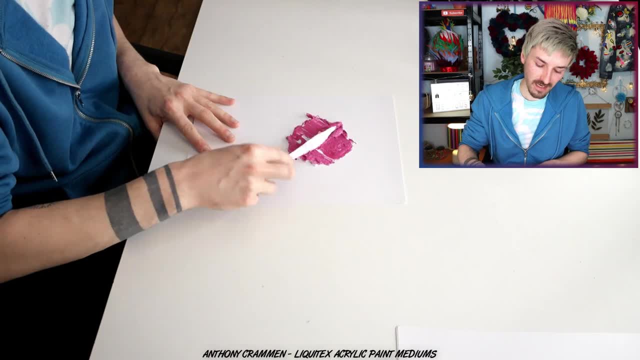 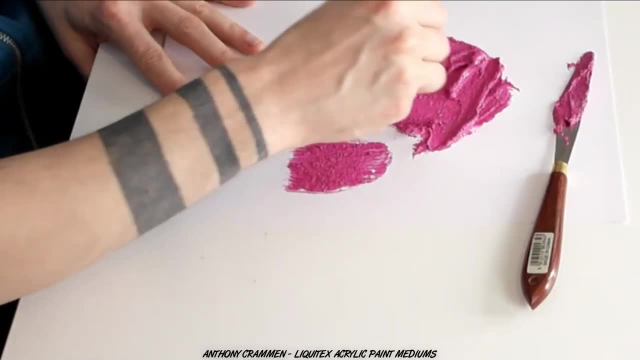 better for building 3d effects than the last one, because I just think it has a bit more of a structure to it. I also think if you're painting kind of beach scenes or something, this one would be quite nice because it does have a really coarse texture. It's not bad, it just feels like I've mixed. 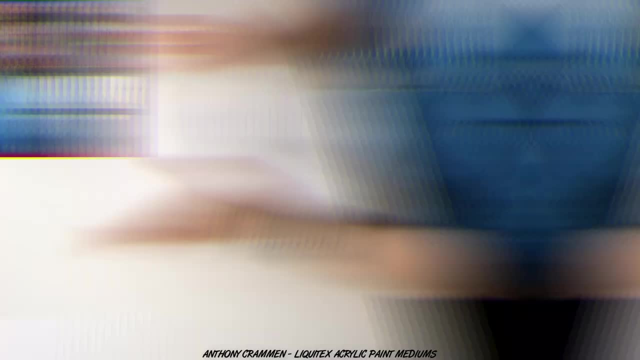 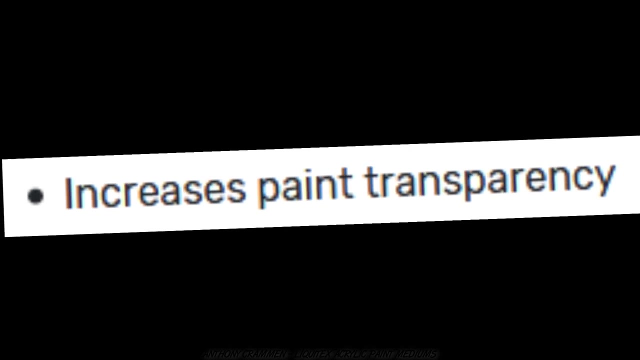 my paint with sand again, But we'll put it to one side and let it dry. Okay, next up we have the iridescent medium and this apparently gives a smooth, iridescent appearance. it increases paint transparency, extends your color without affecting acrylic stability. slows dry in time to help you. 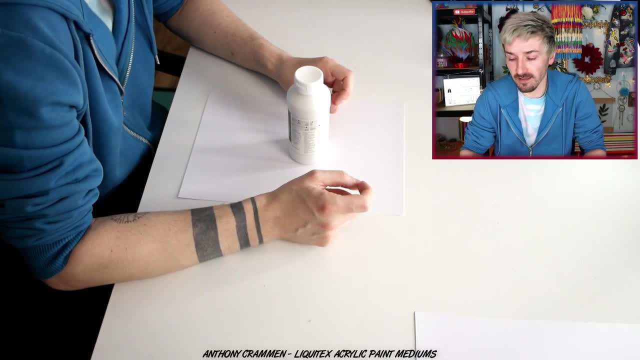 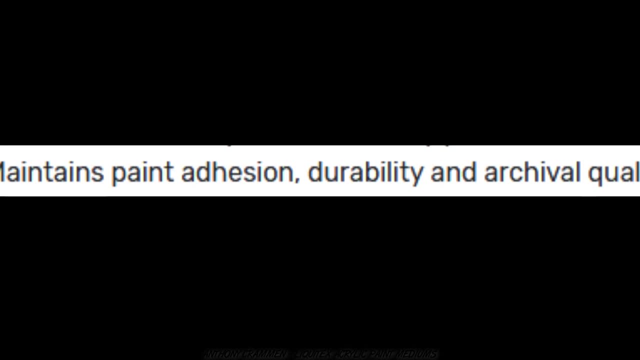 create more subtle color blends, lowers the- I can't say that bloody word- Lowers the viscosity of heavier body paint, and it also maintains paint adhesion, durability and archival quality, like all of them do. Right, let's open it. 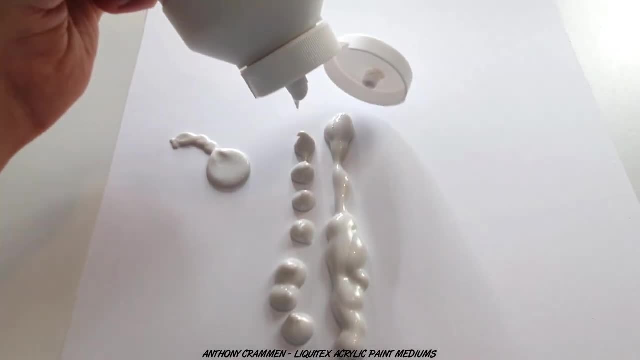 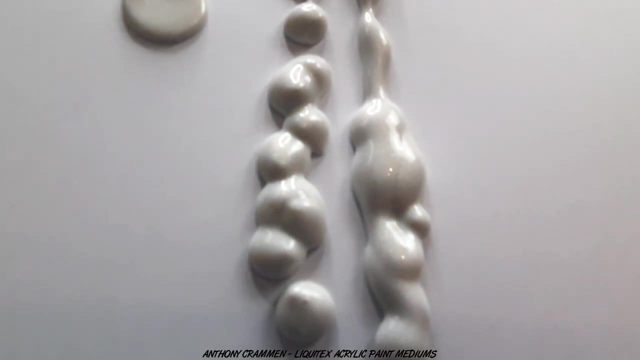 up see what it's like. Okay, and this one is slightly different from the last couple we've tried, because it's more of a paint consistency. it doesn't have a thick gel kind of consistency And on its own it kind of looks silver and pearlized and it's got. 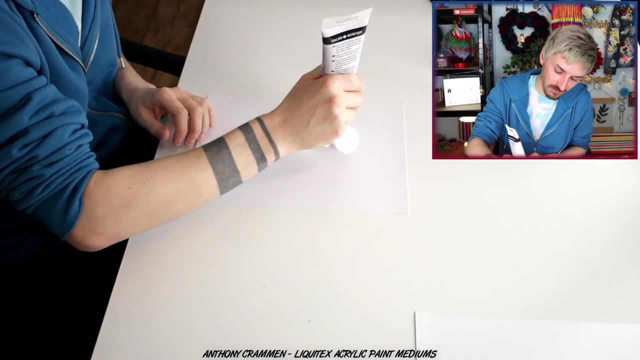 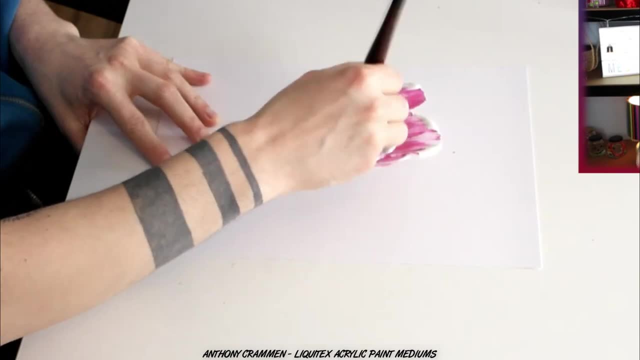 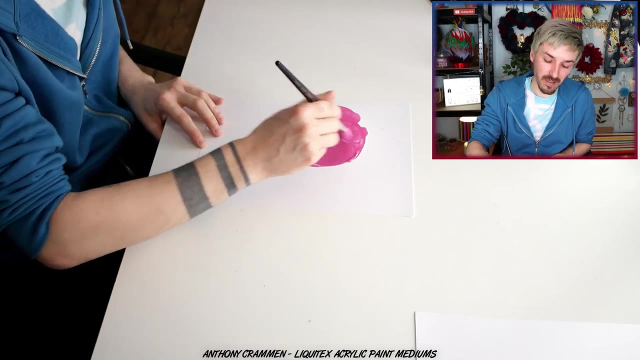 maybe some glitter in. it looks quite nice, Just add some paint to it. It did say that it extends the color without affecting acrylic stability. I personally find that it thins your paint out. it makes it a lot more runny, but it hasn't made it. 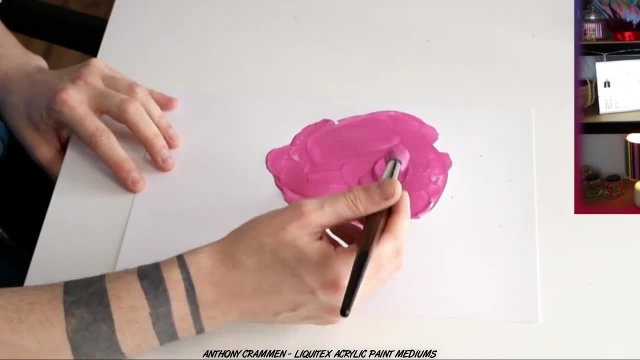 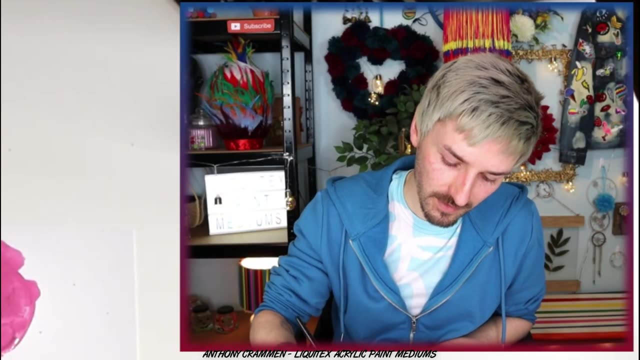 kind of transparent or anything. it does say that it increases paint transparency. For me, I feel like it almost does the opposite. it creates more of an opaque finish, but I quite like it. it's quite nice. The fact that this can turn any paint iridescent is pretty cool, and yeah, it is nice, just obviously. 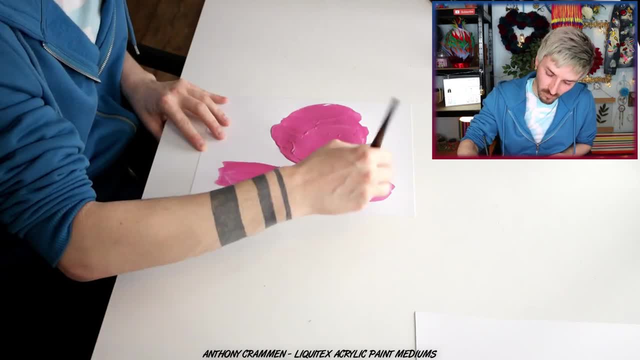 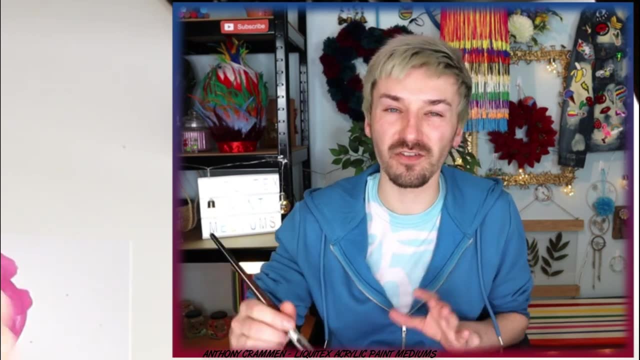 won't thin your paint out a little bit, but it's very smooth, it's got a nice finish to it. You're not going to be able to build texture or layers or anything with this one. it's not something for kind of structure, it's much more of a kind of flat finish. But we'll see what it looks like. 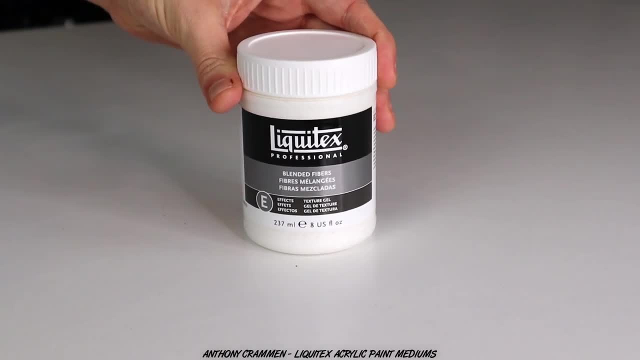 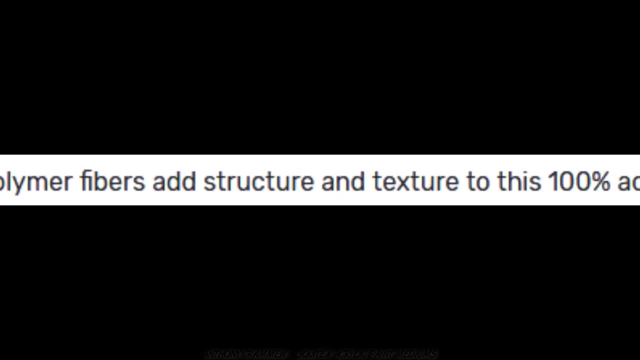 when it's dry. So next up we have blended fibers, and I think this one's quite a strange one. it's very unusual, But it says on the website that a regular size acrylic polymer fibers add structure and texture to this. a hundred percent acrylic polymer gel dries through opaque, matte pull. 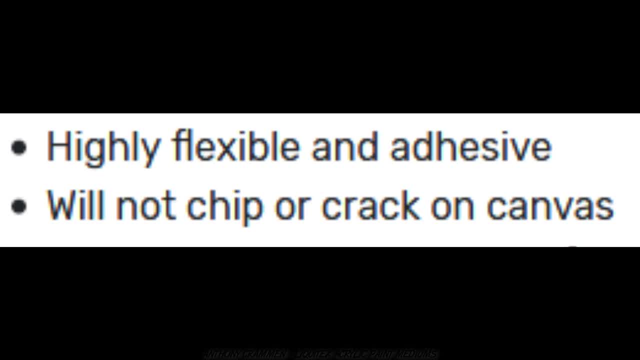 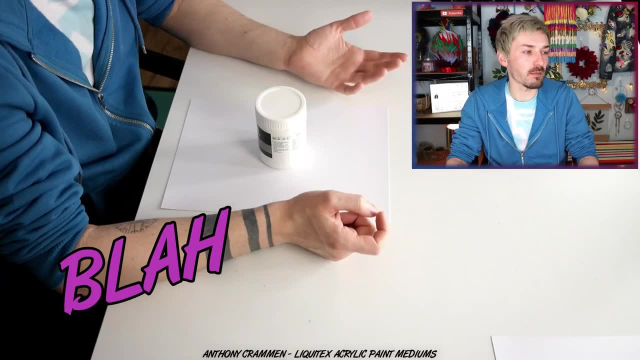 pre-finish. it's highly flexible and adhesive, will not chip or crack on. canvas, holds unusual peaks and knife strokes, a little like textile or organic fibers can be used on its own. blah, blah, blah, yeah, and it's just repeating itself again. Okay, let's open it up, see what it's like. So this 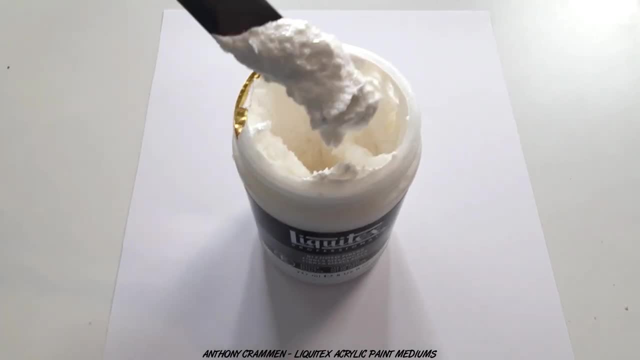 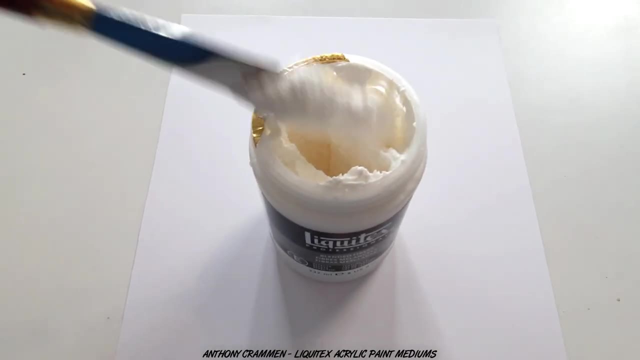 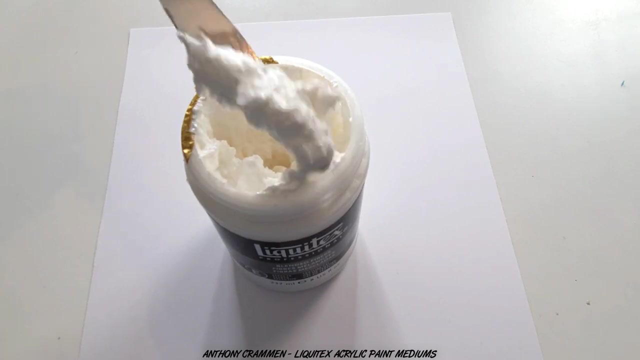 one has a very similar texture to which one was it that we tried The white opaque flake one? it's kind of got like a yogurty, thick, creamy kind of consistency, almost like a mousse. I'm not entirely sure about the fiber part of it- blended fibers, so it's supposed to kind of look like fabric. Yeah, 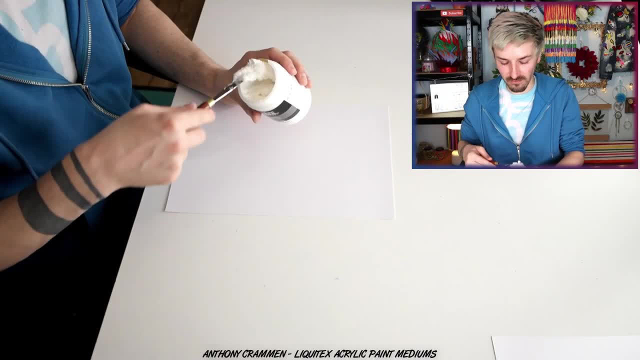 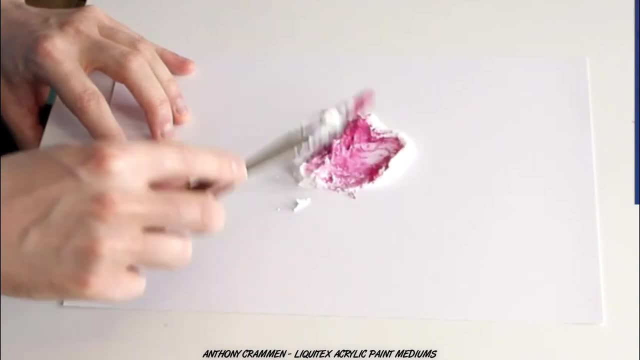 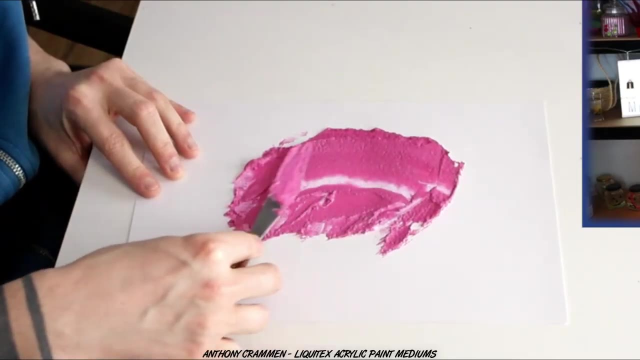 it's supposed to look a little like textile or organic fibers. I don't know about that. See what it looks like with some paint **Music**. So for this one, I'm not sure whether it actually does kind of look textily or like fibers or 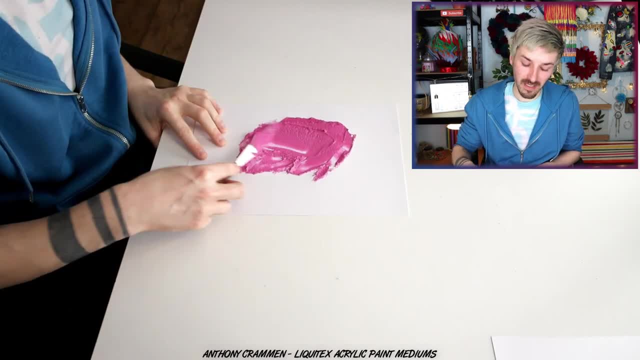 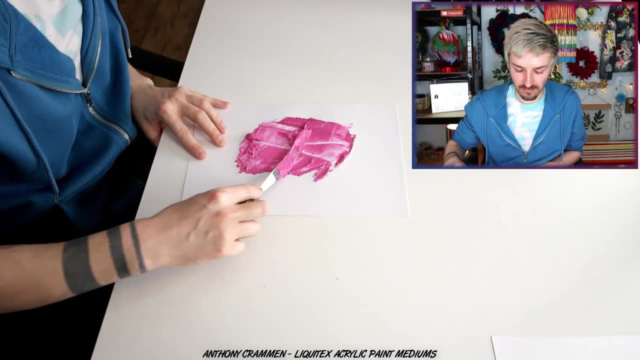 anything like that. It almost reminds me of the thickening paste that they make, but a lot more kind of softer and creamier version of it. You could probably build up quite nice layers with it, but I don't know about this one. Or if it does anything to the paint, it's not particularly. 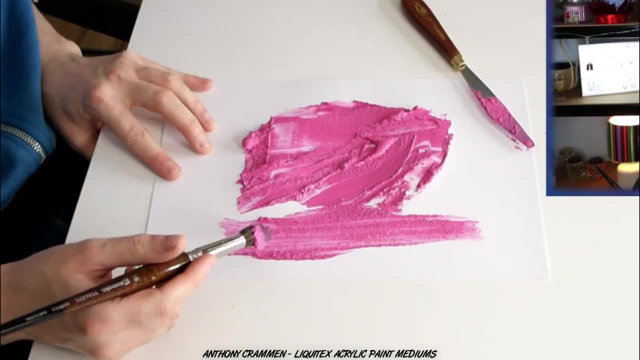 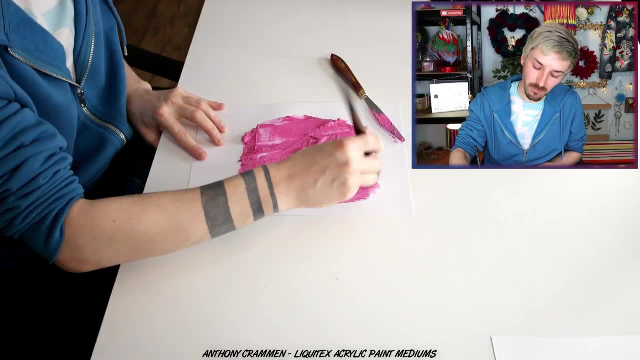 jumping out at us. Let's have a little look with the brush. Now. I wouldn't say it looks like fibers or fabrics or anything like that, or that. it has a textile kind of finish to it. When you use it with a paint brush it's got a very similar texture visually to the sand- not obviously. 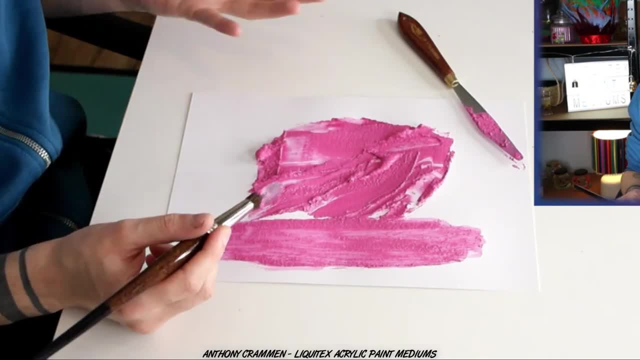 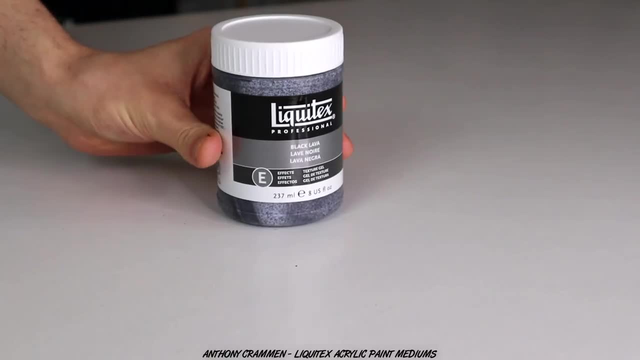 to the touch And with a spatula. again, it just looks kind of like a thicker acrylic paint, But we'll see what it looks like when it's dry. So, last but not least, we have black lava, and this one has to be the most unusual paint medium out of the lot of them that we've tried. 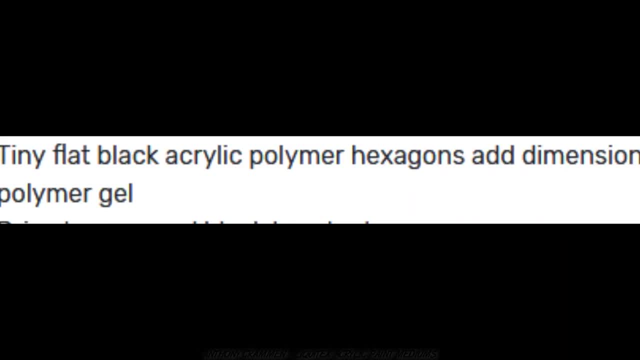 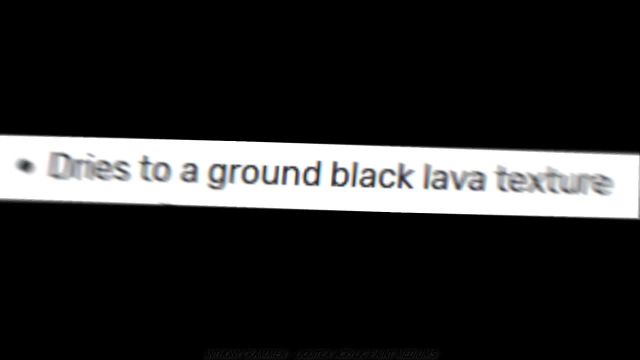 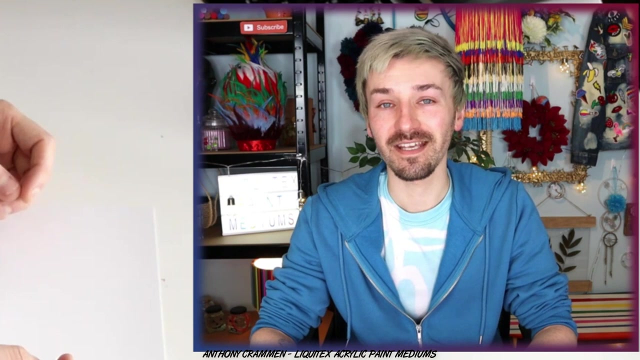 so far it's very, very different. It says on the website that tiny flat black acrylic polymer hexagons add dimension and texture to this clear, 100% acrylic polymer gel. It dries to a ground- black lava texture. what does that mean? Black lava texture? I'll have to take their word for it. 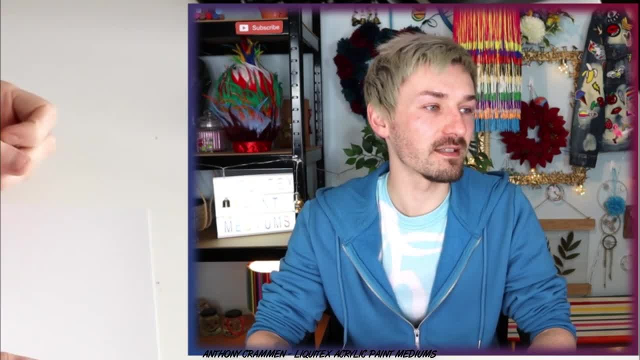 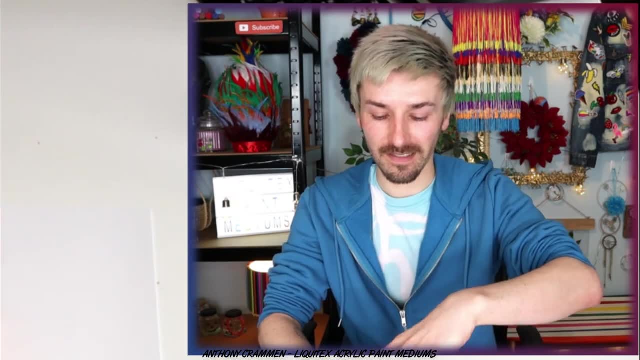 because I've never seen black lava in person. It's highly flexible and adhesive and it- yeah, it- just repeats itself again. They just write the same thing for all of them. Right, let's open it up, see what it's like. 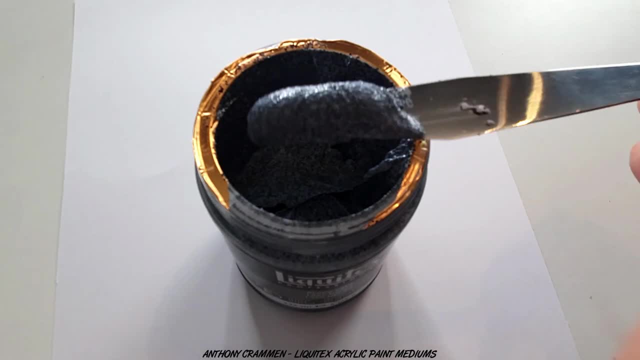 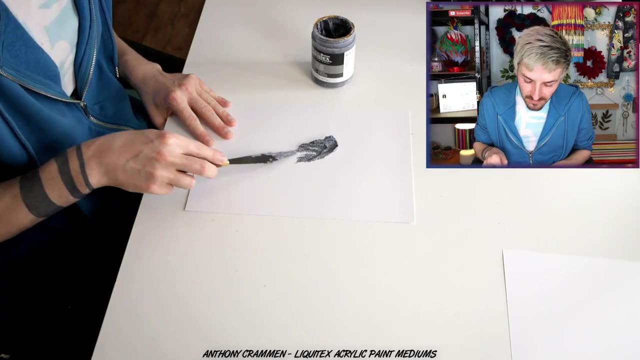 So with this one you've got more of a darker color. it's kind of like a very dark gray and it's quite thick. It's more of a paste consistency than a gel. So I'll pop some on see what it's like. You definitely can see all those little tiny little black bits in there. 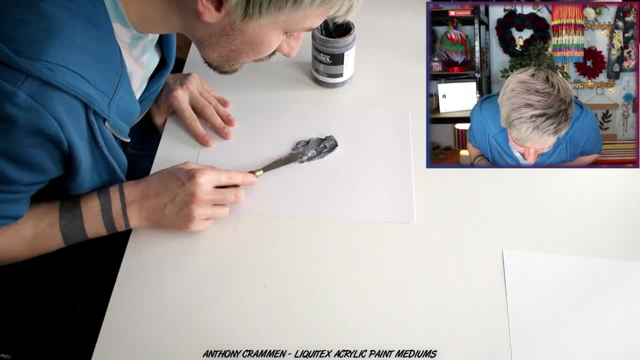 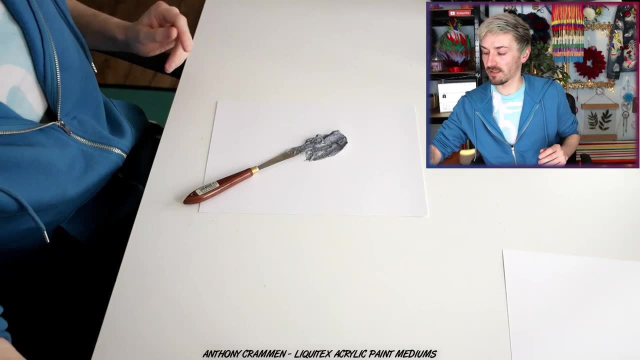 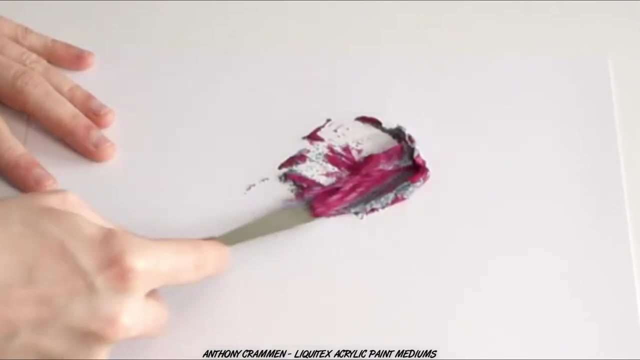 It says that they're hexagons but they look like circles to me just saying It kind of looks like frog spawn a little bit. it's very strange. Let's add some paint to it, see what will happen. **Music**. 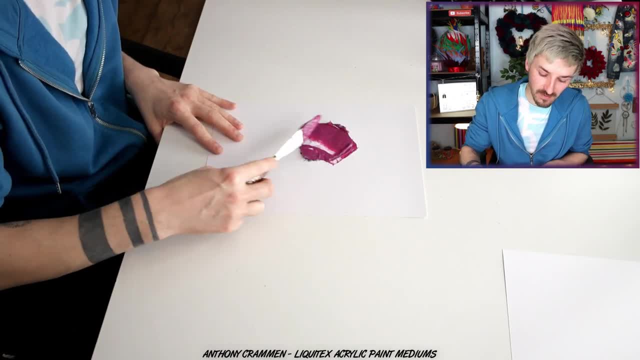 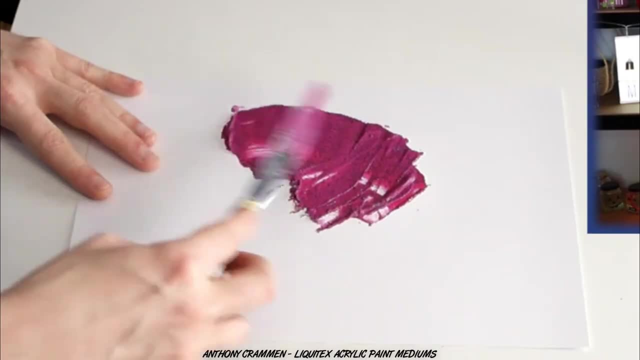 Okay, it definitely darkens the color of your paint and you can really visibly see all those little black dots in there. It is quite interesting. I think it would be quite nice for some abstract paintings to add just a little bit of detail, a little bit of texture. 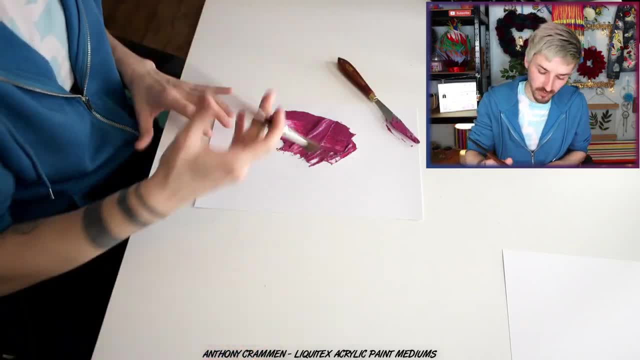 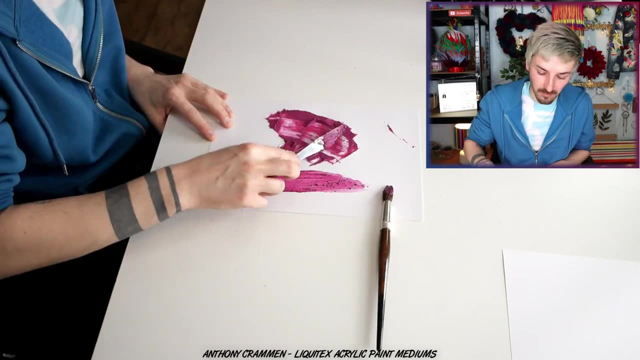 maybe even some figurative paintings as well. Let's have a little look with the brush. it almost looks like you've got like bits of dirt in your paint when you use a paintbrush with it. I think I prefer it with the spatula and kind of build up layers. that way I think I like it the most, because it's just very. 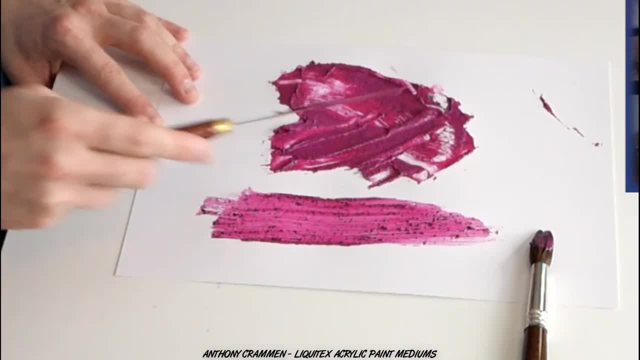 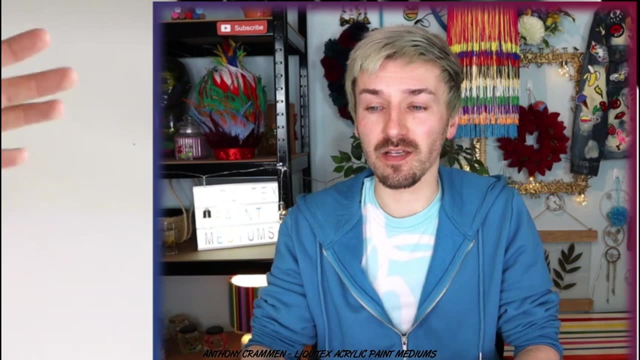 different. it's not something I've seen before, But I'll be interested to see what it looks like when it's dry, see what the finished effect looks like. So we'll pop that to one side. So I did use all of these mediums about a week ago so I would have some dry samples to show you. But before I show, 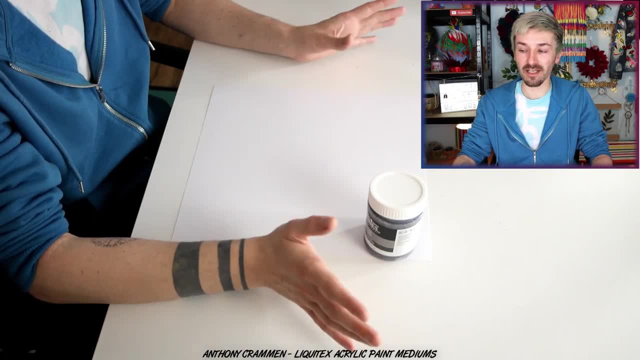 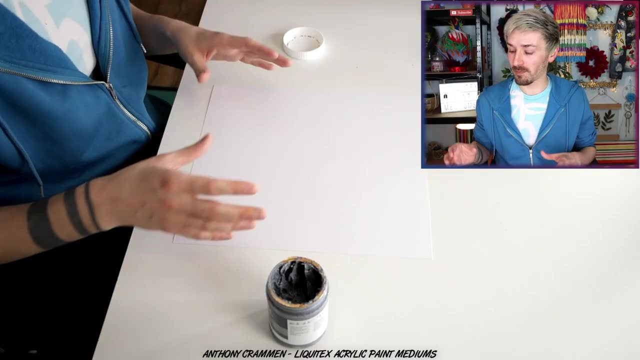 you them. I thought what would be quite interesting is to mix all of these up together just to see an idea, some inspiration. So I'm just going to put all these onto the paper together, mix it with some paint and just see what happens. So pop some blended fiber down. 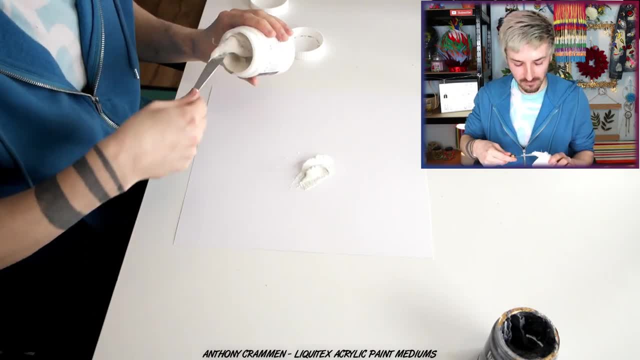 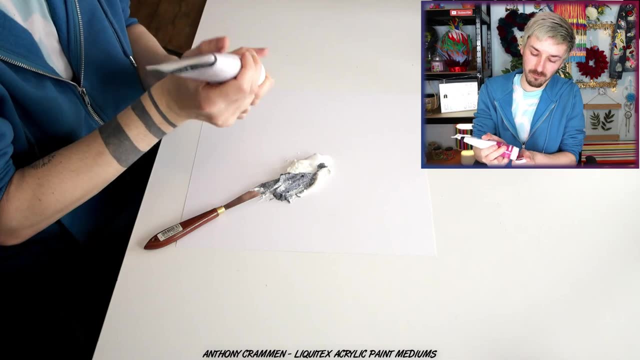 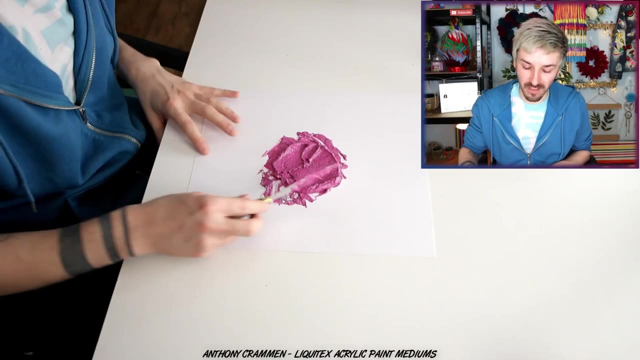 pop some resin sand on some natural sand, some white opaque flakes, some of the iridescent medium and some of the black lava as well, And we'll pop some paint in and see how this turns out. Strangely enough, one of the mediums has kind of knocked the thickness out of it. 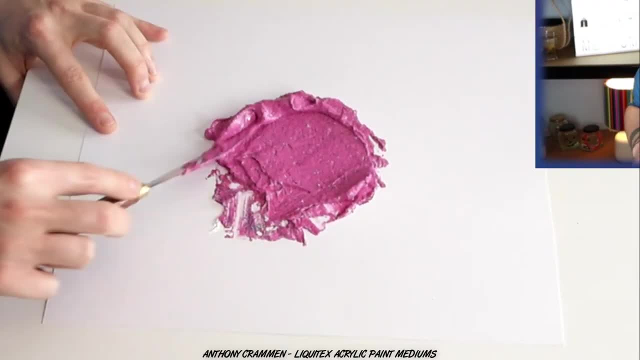 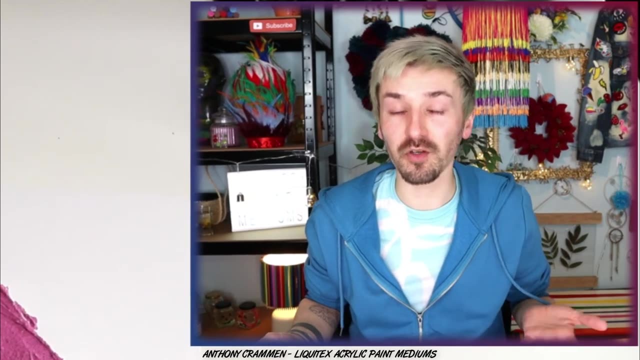 so it just kind of flops back down, But the black lava you can definitely see. I'm just wondering whether it'll turn iridescent. I'm quite curious to see what this will look like when it's dry, but obviously I'm not going to have time to show you that in this video. 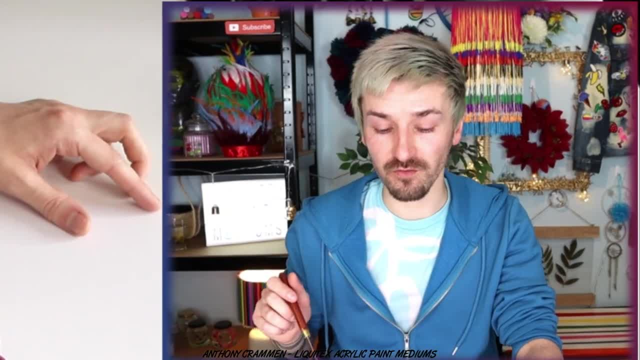 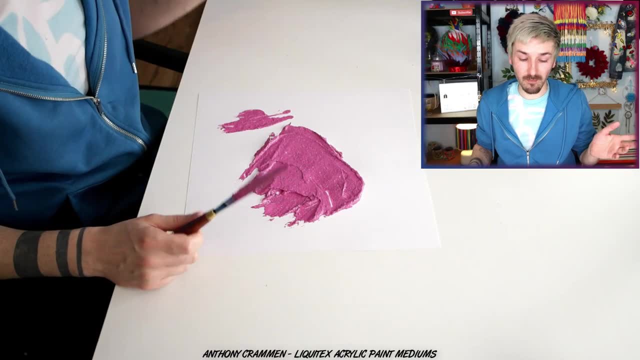 But what I will do is I'll post this on Instagram once it's dry, so make sure to go follow me on there, and then you can see what this turned out like. Anyway, I'll go get my other samples and show you them and see what the finished mediums look like. Okay, so I've got the white. 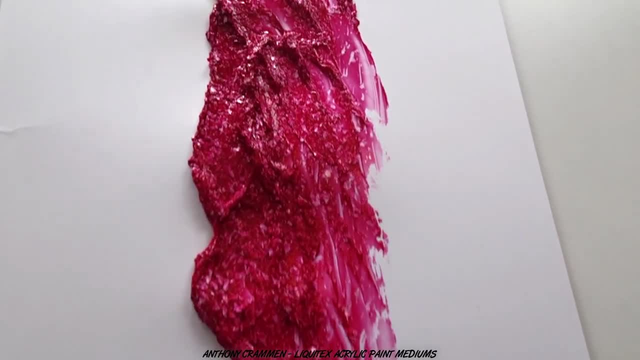 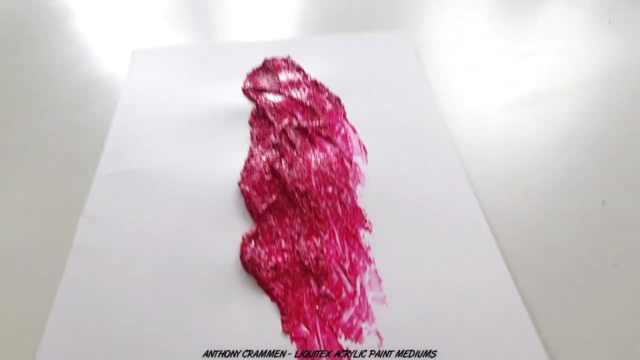 flake one here and it's turned out quite nice actually. it's got a very glossy finish to it and you can definitely see the white flakes they have shone through And it's got a lot of texture. it's very rigid. 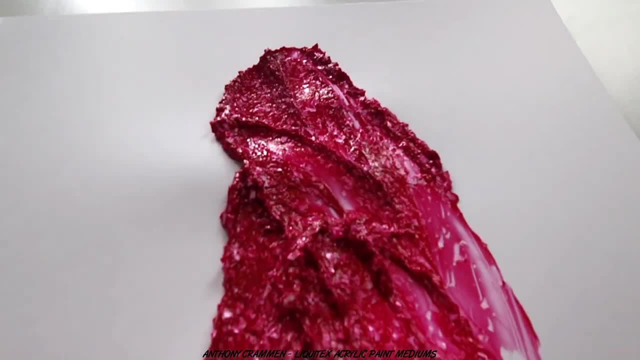 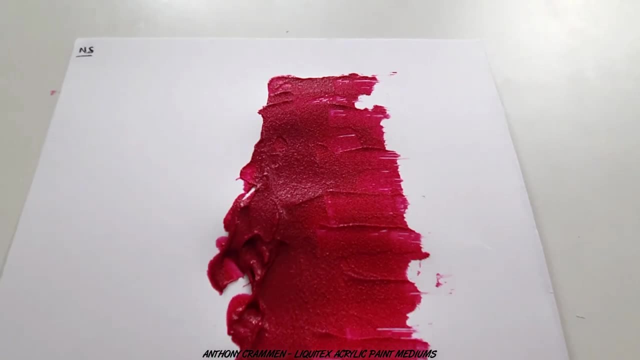 it's very kind of thick and hard, but quite flexible at the same time. It's not bad. actually, I quite like that one. Next up we have the natural sand and again it's given it quite a glossy finish. It's built up some nice layers, it's got a very subtle texture to it and it's quite flexible. 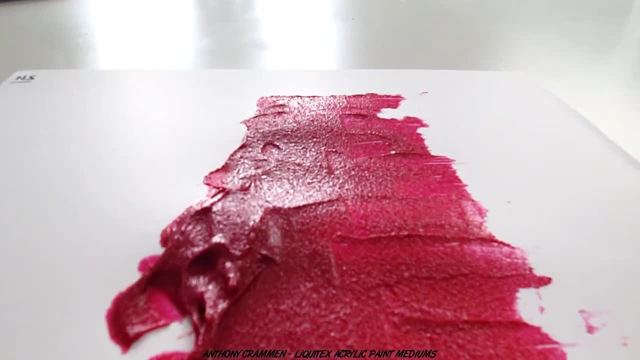 it's not really hard or anything like that. you can kind of see it, It's not really hard, it's not really hard to see, it's not really hard to see and kind of push it around and move it It's, it's not bad. 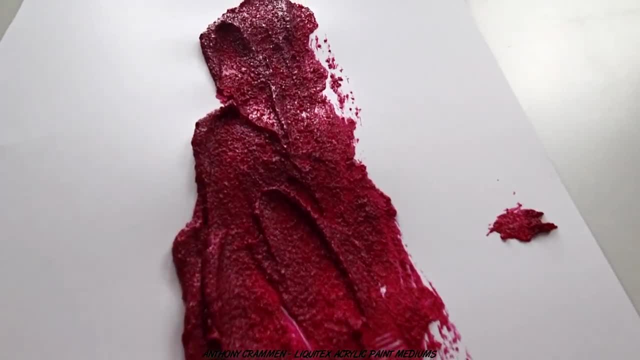 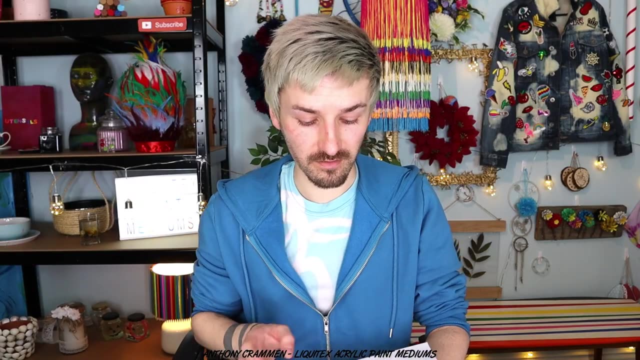 The resin sand has definitely darkened the paint a little bit and it's a lot more rougher to touch, And again you've got some really nice built-up layers and some nice textures there as well, so that's not too bad. The blended fibers has given the paint quite a matte finish. 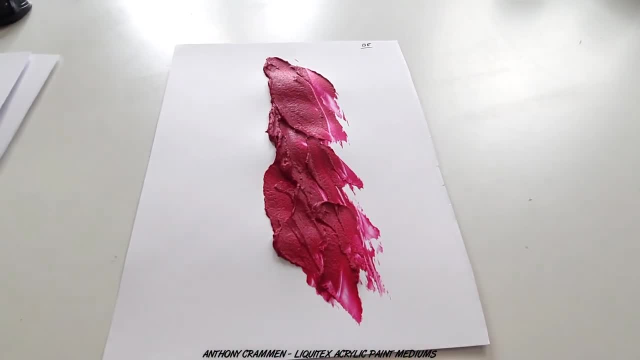 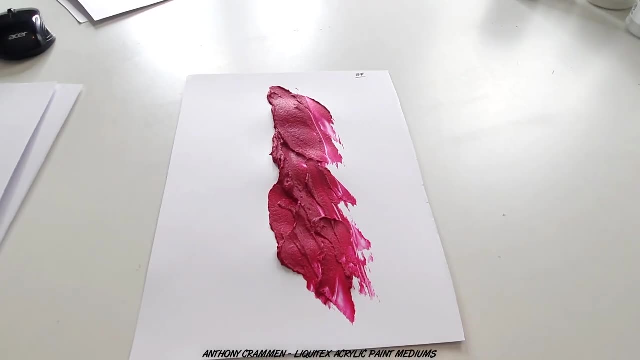 I'm still not sold on whether it actually makes it like fibery or fabric-like or textile-like, but it's done something to the paint. it's definitely thickened it up and it kind of is what it is. Really, I really like the iridescent medium. I think this one's turned out really nice and it's. 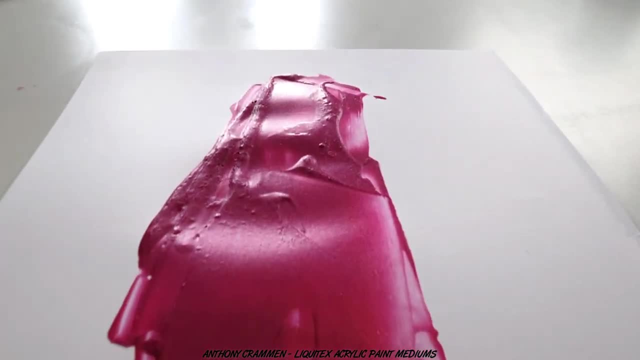 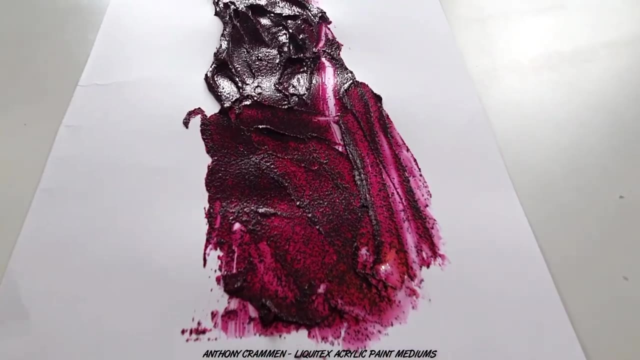 got a really nice shine to it And, like you can see, you probably won't be able to build up a lot of texture with this paint medium. it's much more of a smooth application, But it's really nice. I quite like that one. And then finally we've got the black lava and that's given the paint a very